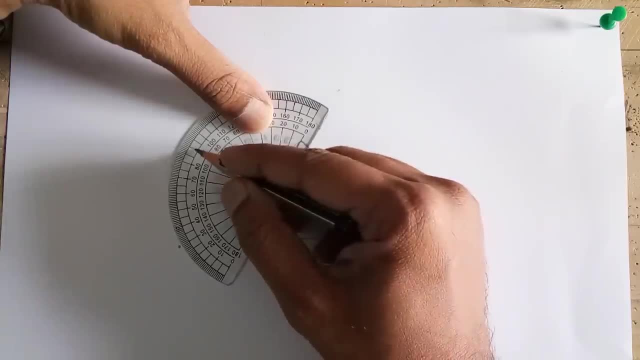 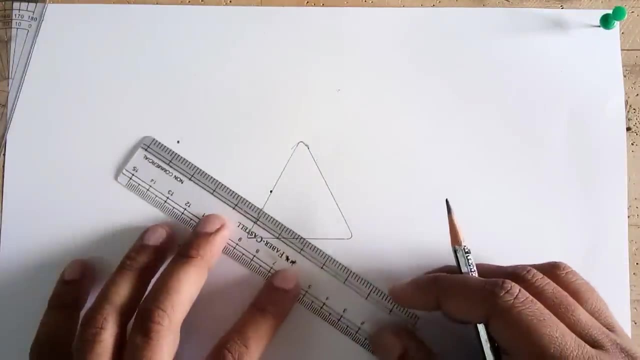 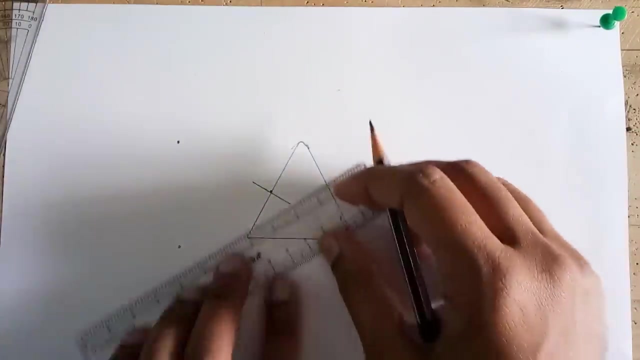 measuring the angle from here. otherwise it would be 30 degree. We are measuring the angle from 90 degree to 30 degree. that's why it is 60 degree. We mark a point on 90 degree as well. Now, this would be your normal and this would be. 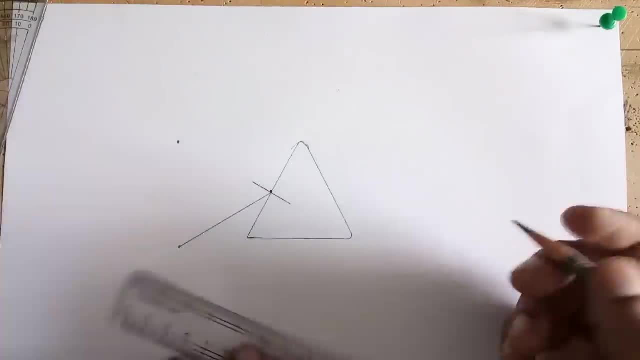 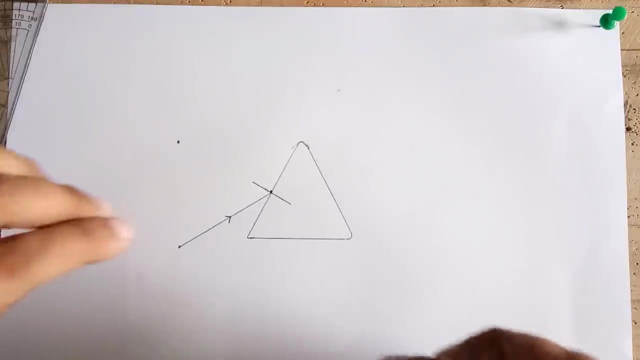 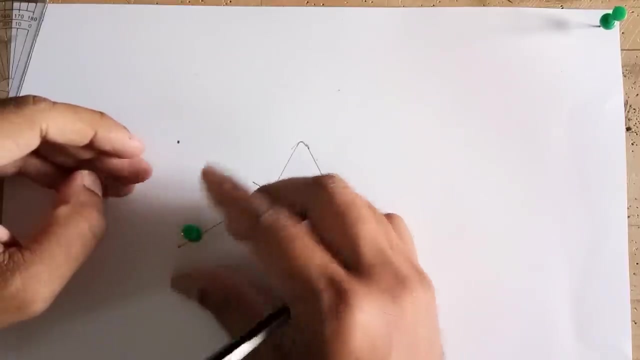 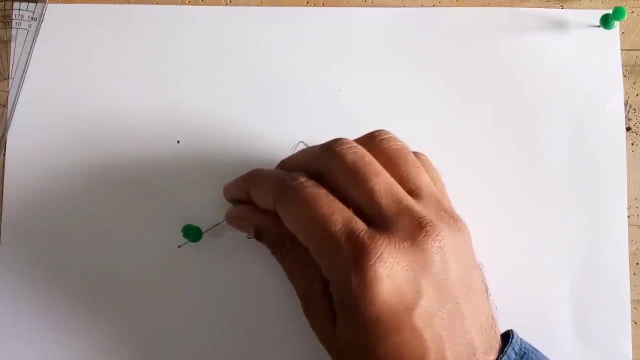 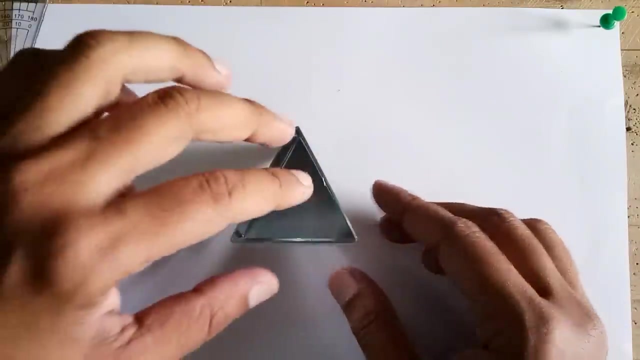 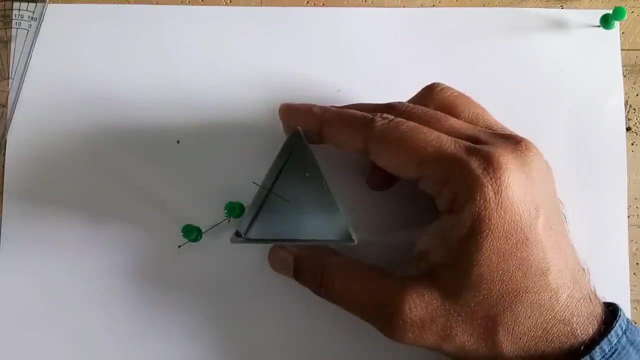 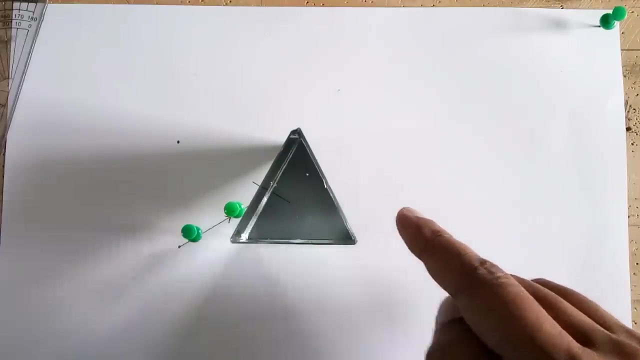 the angle of incidence, right. Okay, Now two pins. you are supposed to fix it over here on the incident ray. Now put the prism back over here at its mark position. Now you are supposed to see these two pins from this side. They will be visible to you, And now I will be seeing the pin on. 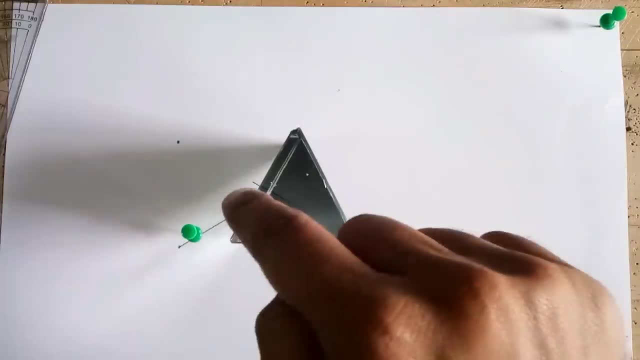 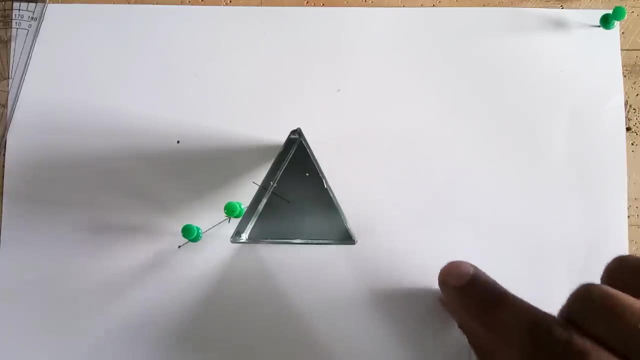 this side, because this is the incident ray, that would be the refracted ray and the emergent ray would be somewhere over here. So I need to put, I need to see the pins from here And you need to see it very carefully with one eye closed to avoid the parallax error. 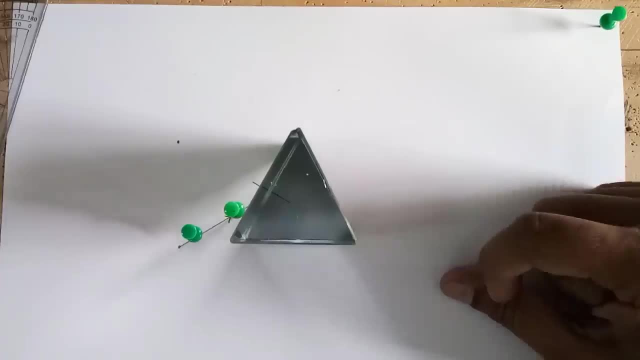 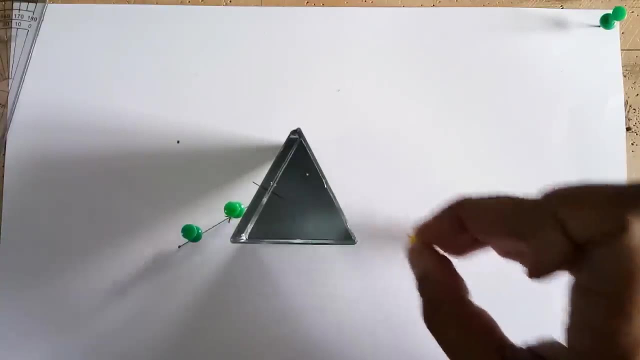 So let me do it, And afterwards what you are going to do is, when you see these two pins over here, we have another two pins which we are going to put it on this side, And we will make sure that these two pins are in straight line arrangement with these two pins. 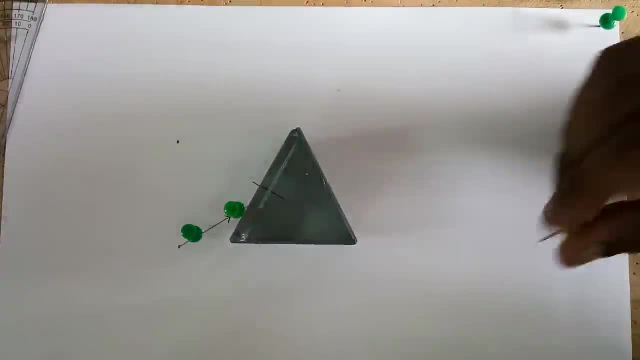 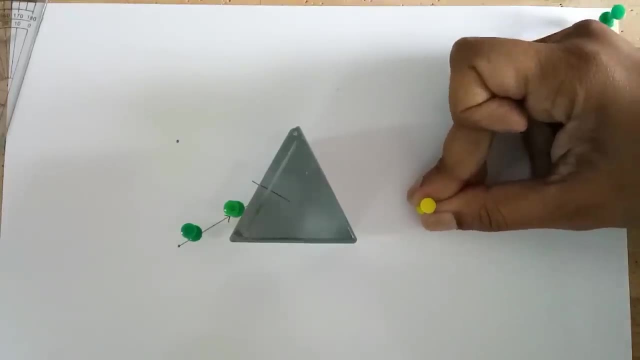 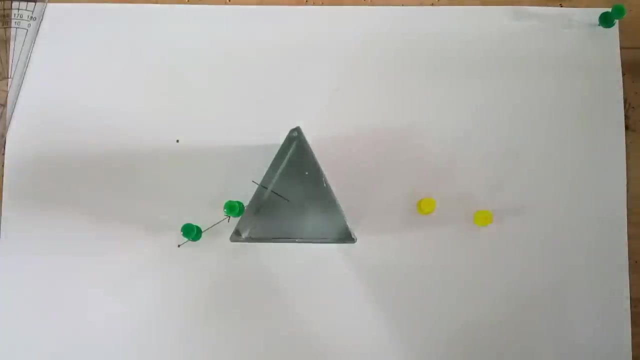 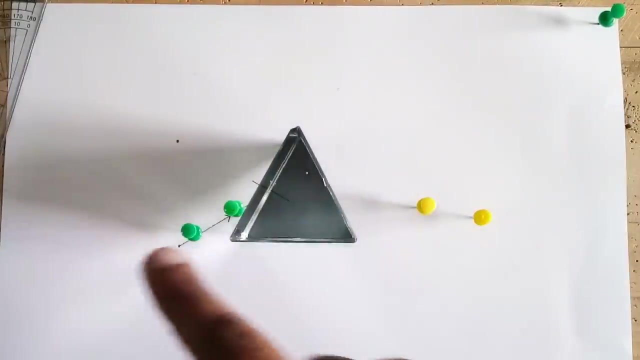 So at these two pins from this side, because this is the emergent ray which is coming to my eye. 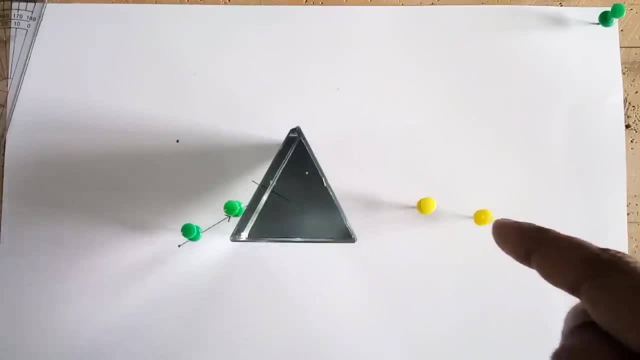 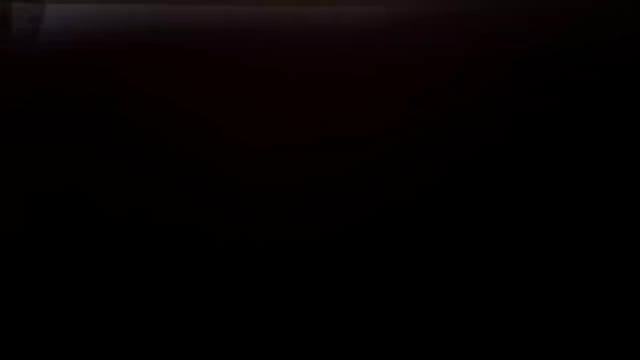 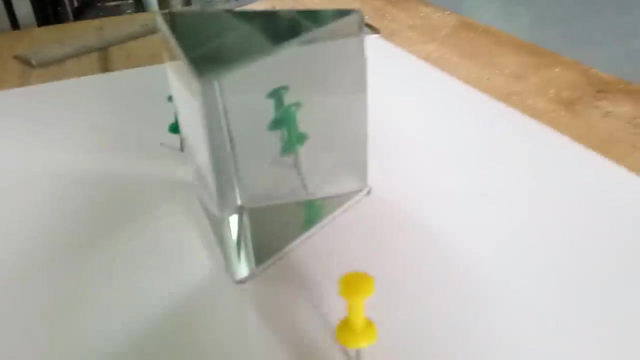 so i would be seeing these two pins in this line, this line and now these two pins i have attached in such a way that all these four pins are visible in a straight line. let's see it. so if you watch, if you, if you watch, these two pins, these two green colored pins, are visible. 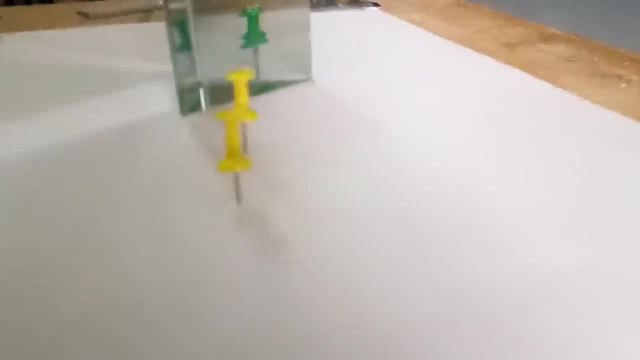 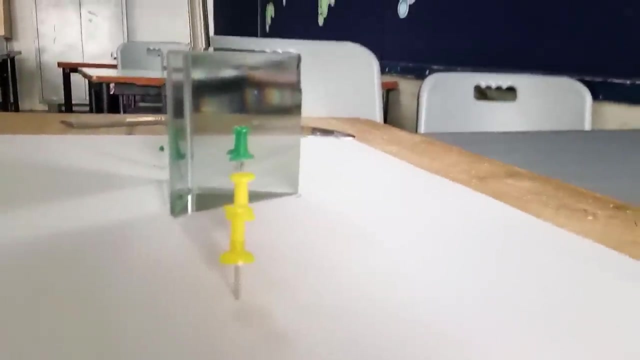 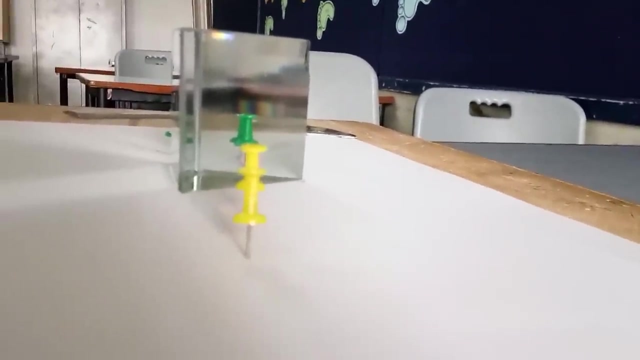 over here right and now. if you see that all four pins are appearing in a straight line, you guys are lucky because you can see the spectrum band of seven colors at the back side. so you can see very carefully. all four pins are placed in a straight line and quite spectrum is. 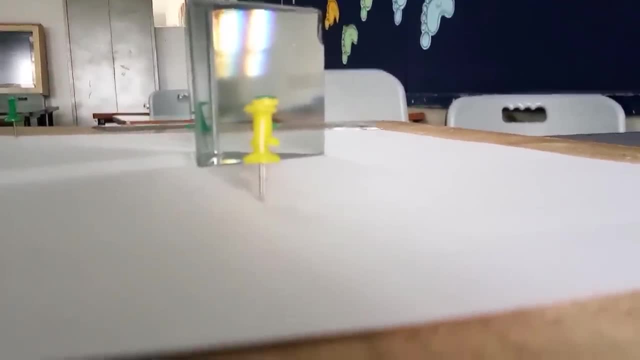 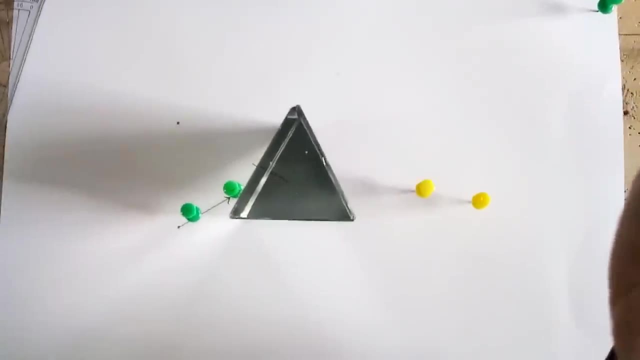 visible. on the top part you can see that there is a spectrum, so dispersion is also seen over here. right, okay, okay, okay now. what we are going to do is: now we are going to mark these two, these two places. so i'm going to remove these pins. 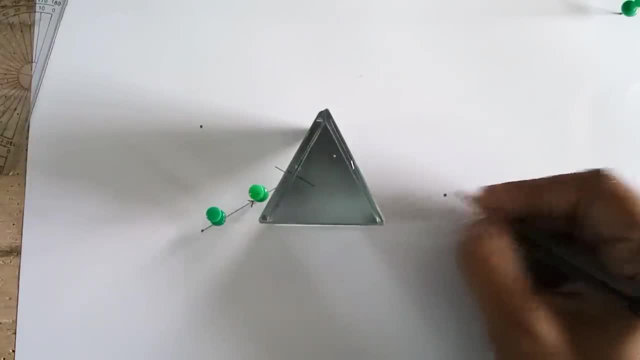 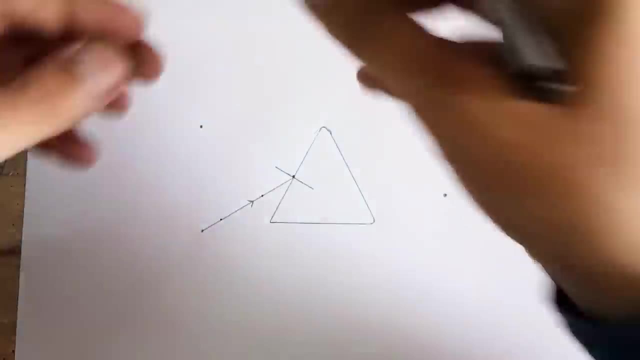 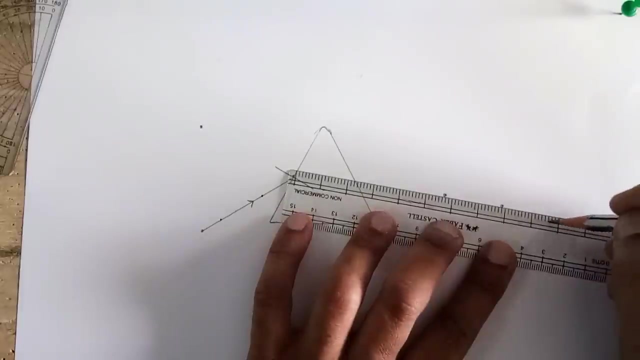 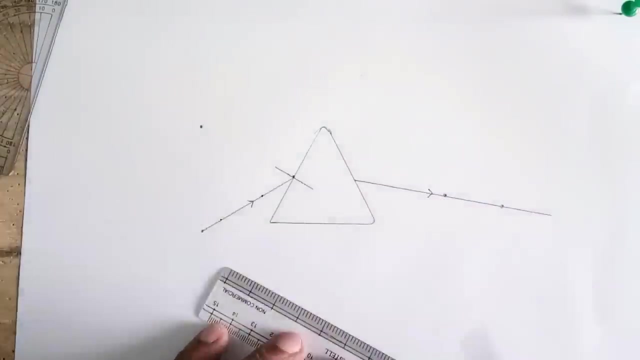 now we'll put the prism aside. okay, now no need of these pins. also, these two points join with the straight line over here. this will be your emergent ray, and from here the normal is at an angle of 90 degree, so this will be the angle of emergence. this is the angle of incidence. 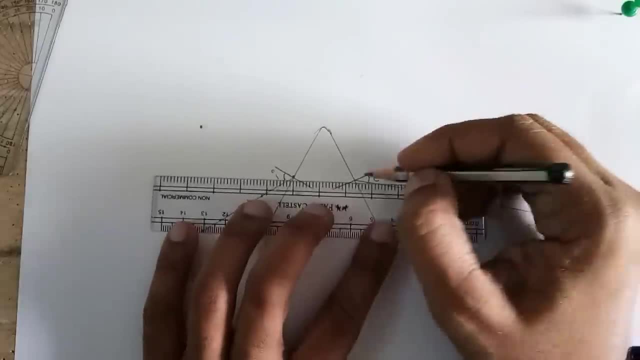 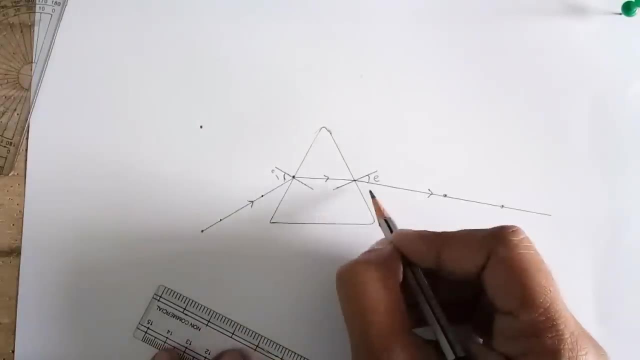 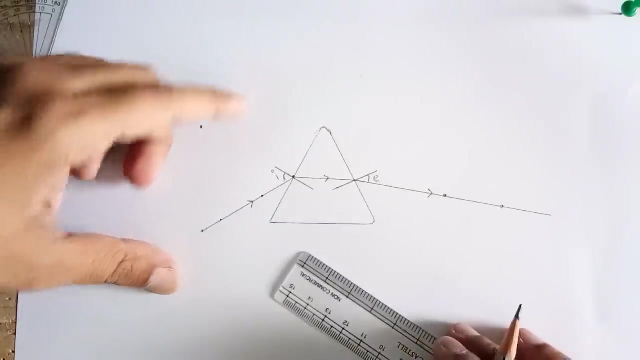 this. Now I am going to join these two points, and this would be my refracted ray, Incident ray, refracted ray: now you can see that it is, instead of going straight, it is bending towards normal due to the refraction. Now our main task is to find the angle of deviation. 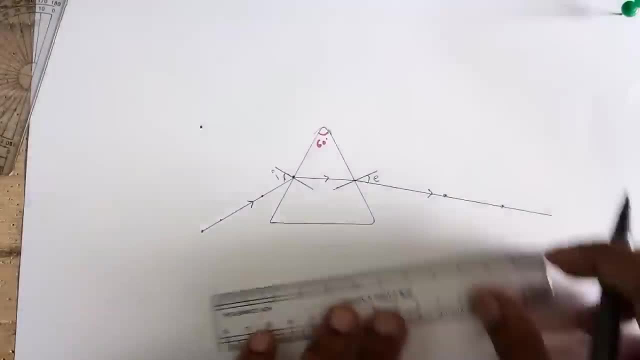 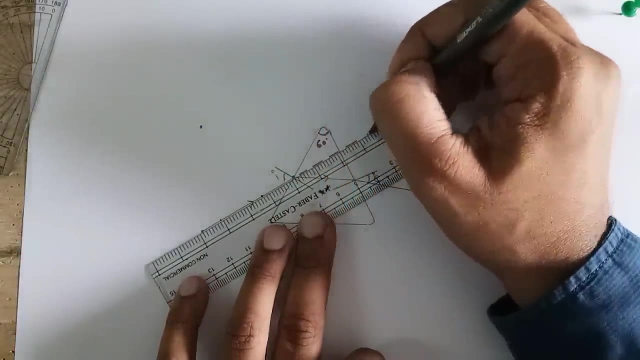 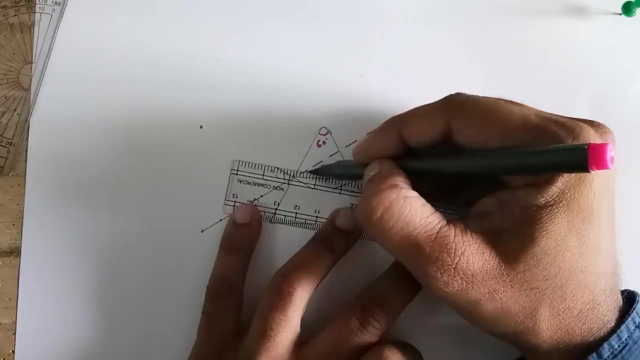 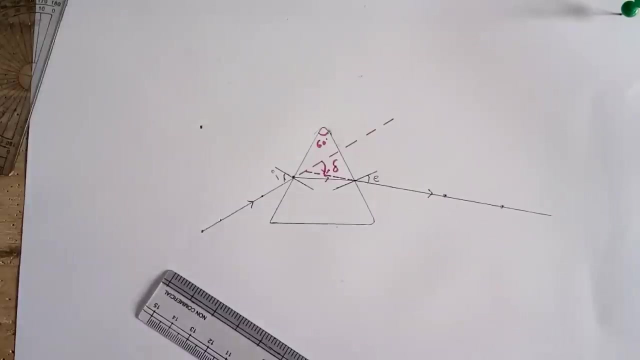 We know that this angle is 60 degree right angle of prism. Now I am going to extend the incident ray forward and I am going to extend the emergent ray backwards, So I get this angle that is called angle of deviation. So let us measure with the help of a protractor. 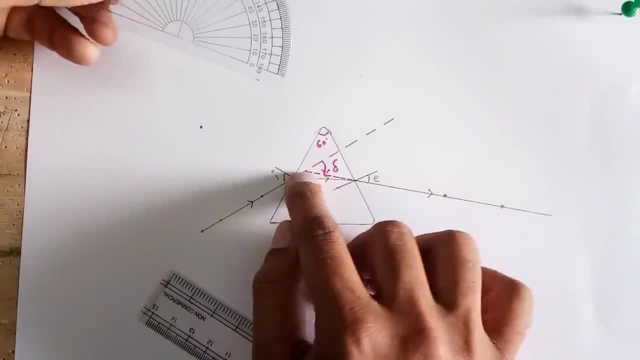 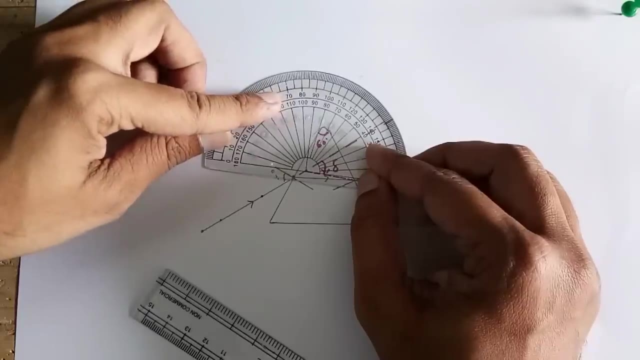 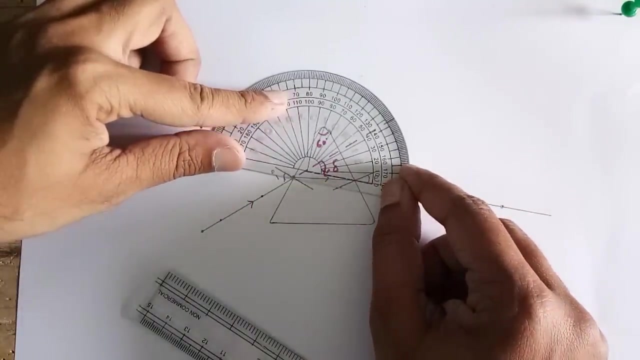 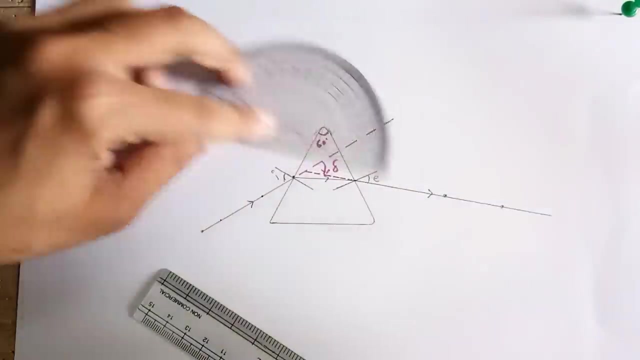 Okay, how do you measure this? See, make sure that this point is falling over here. So, like this: And the angle of deviation: this line matching with this line and the angle of deviation is just over 40 degrees. It is approximately 42 degrees. So the angle of deviation for 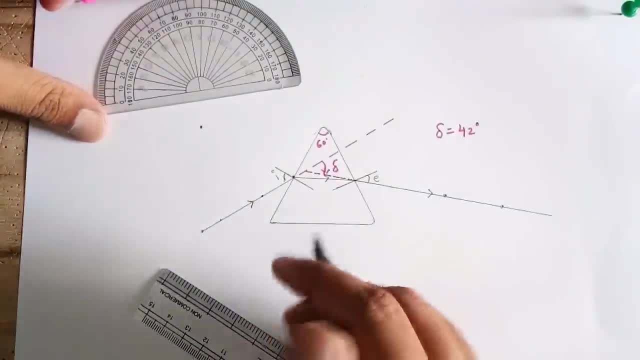 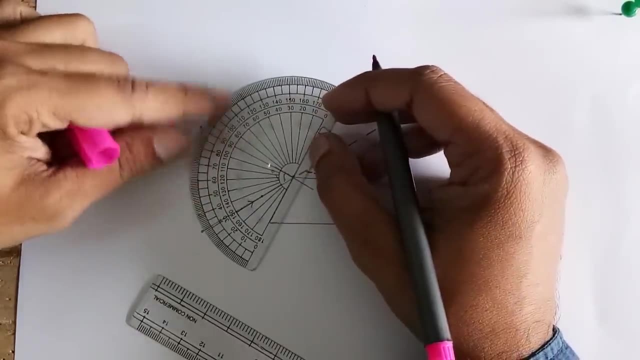 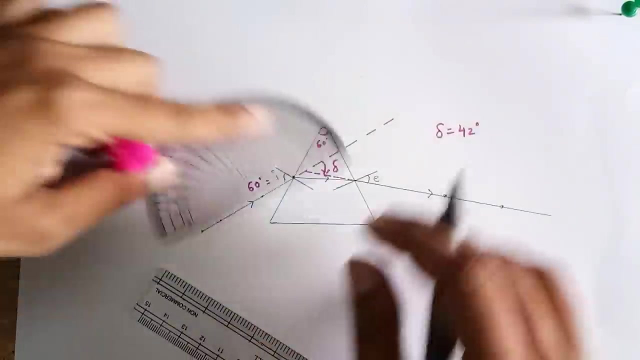 the prism is 42 degrees right And I kept the angle of incidence as 60 degree. If you just want to measure The angle of incidence, I had kept it 60 degree. So when I kept this angle, 60 degree, I got the angle of deviation is this. Let me measure the angle of emergence as well. So angle of 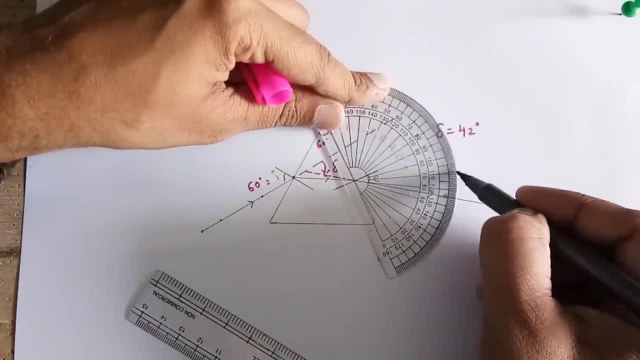 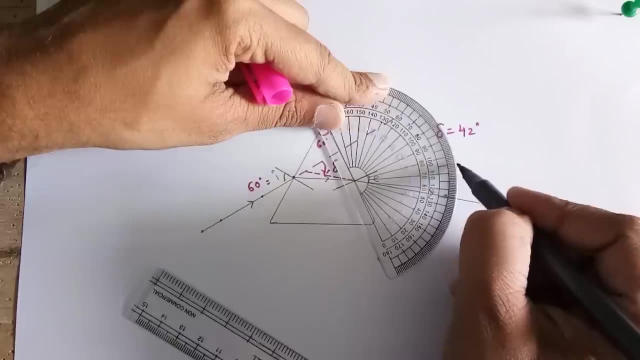 emergence with respect to the normal 10 degree, 20 degree, 30 degree, 40 degree. You can see that from here. 90 degree, this is 10, 20, 30. Now, I am mistaken, it is. yeah, it is the same. 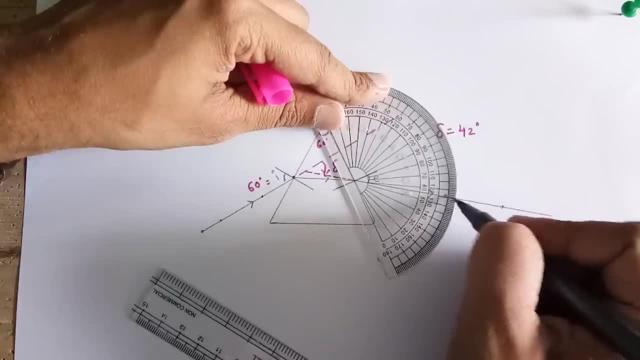 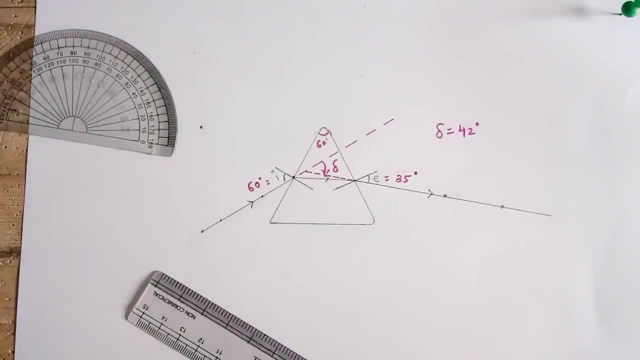 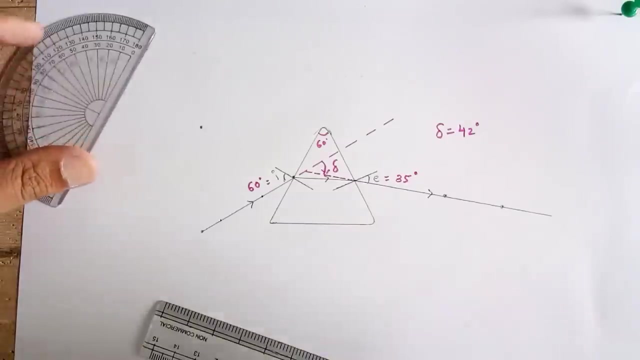 only 40. No 35, sorry, because this is these are the gap of 5.. So this angle is 35 degree, right? So this was the experiment about the dispersion, sorry, the refraction through prism. Hopefully you have understood this. If you have any doubts, you can comment in the doubt section. Thank you for watching the video. 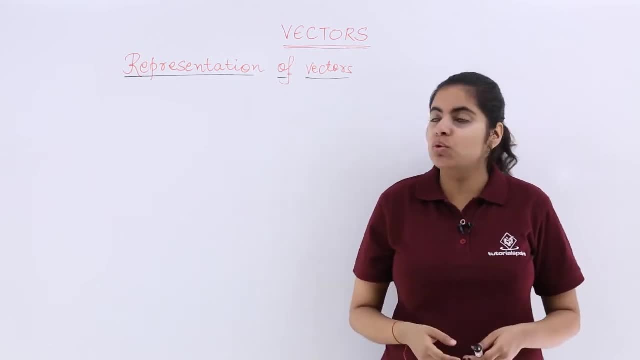 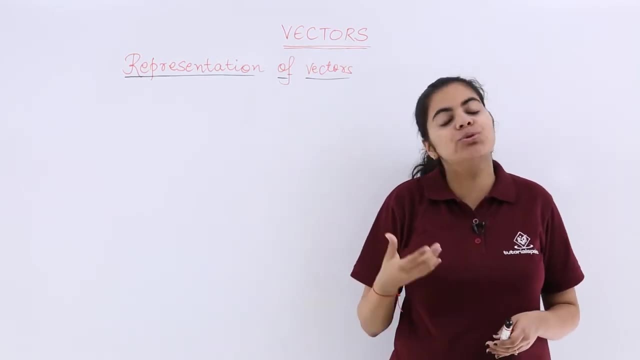 When you know about what are vectors and what are scalars, let's move into the representation of vectors subtopic. Now, as you see, it says representation of vectors means how do you show or depict or represent your vectors. So vectors, as you know, should have both direction.